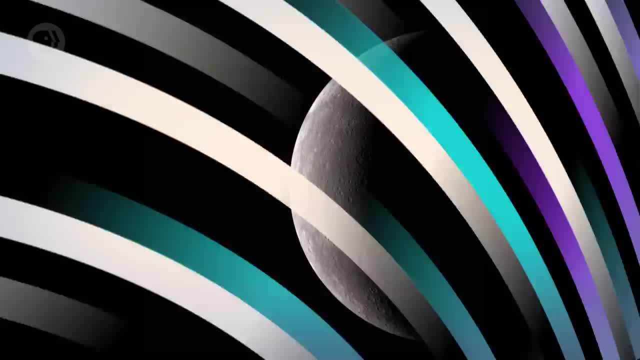 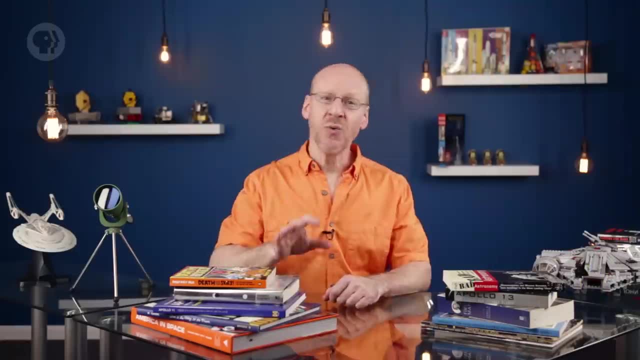 In 1639, the Italian astronomer Giovanni Supi used a telescope to observe Mercury, and he discovered it undergoes a complete cycle of phases over time, just like the Moon does. The only way that can happen is if Mercury orbits the Sun and not the Earth another. 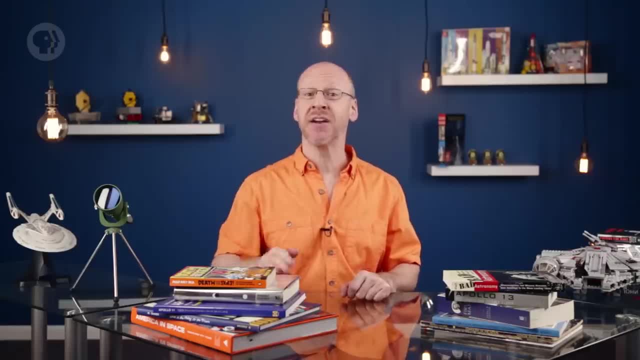 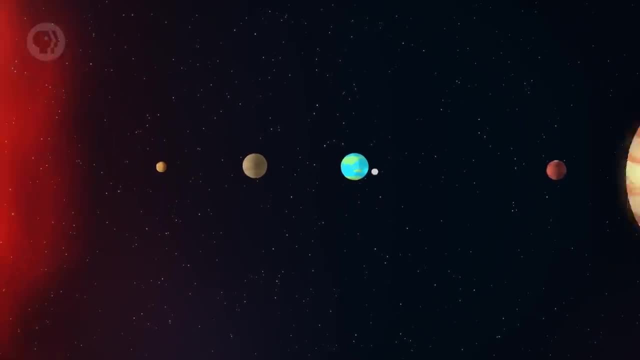 checkmark in the column for heliocentrism, which was starting to look better and better all the time. And of course, that's the way things really are. Mercury is the innermost of the planets in the solar system. It orbits the Sun at an average distance and the Sun orbits the 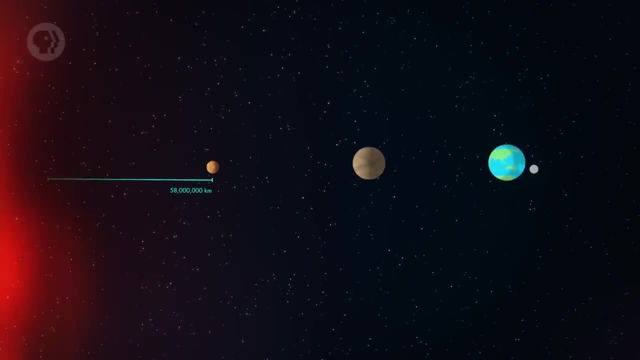 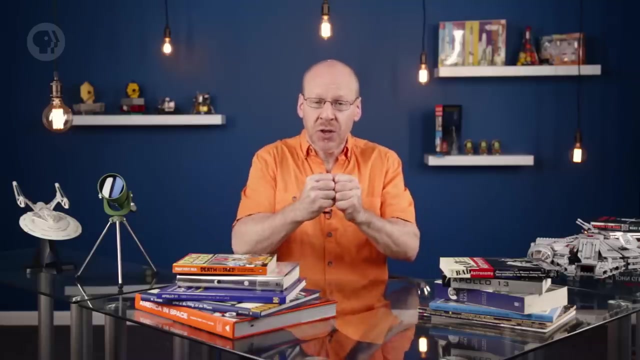 Earth at a distance of about 58 million kilometers, roughly a third the distance of the Earth from the Sun. That's why we never see it stray far from the Sun. From our viewpoint, its smaller orbit keeps it huddled closer to our star. That's why we see it move. so 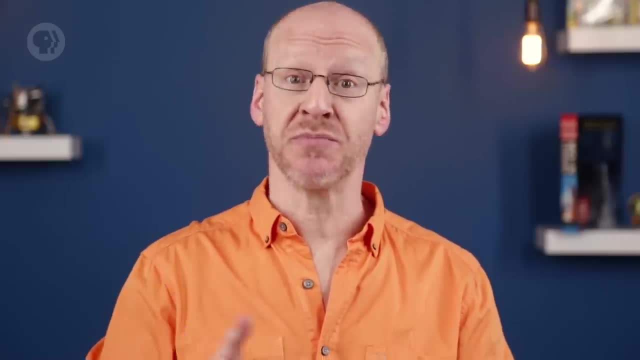 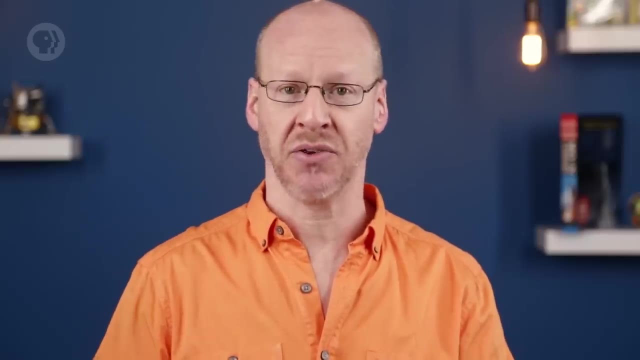 rapidly too. It's closer to the Sun, so the gravity it feels from the Sun is stronger, and therefore its orbital velocity is faster than Earth's. It orbits the Sun once every 88 days, And that's also why we see it undergo phases. 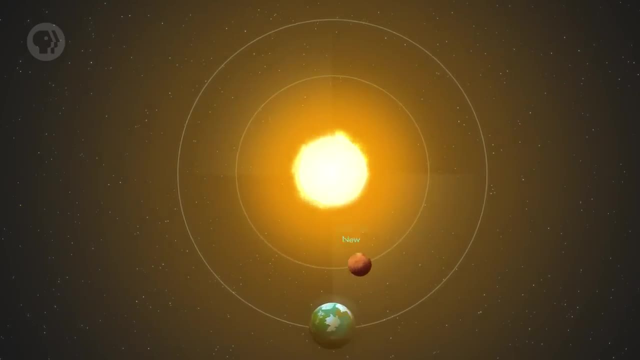 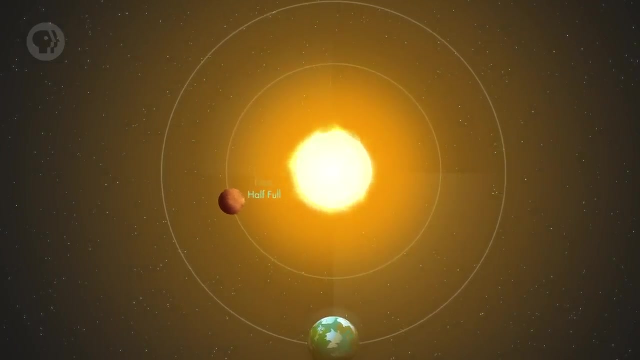 When it's between us and the Sun, we're looking at its dark side, and when it's on the other side of the Sun, we're looking at its fully illuminated half. In between, it goes through the same phases as the Moon – crescent, half-full, gibbous, and so on. Not that this is such. an easy observation to make, Because it never gets far from the Sun. it's always low to the horizon after sunset or before sunrise. When we observe it, we're looking through all of the muck and turbulence in our air, so it's usually pretty fuzzy Making matters. 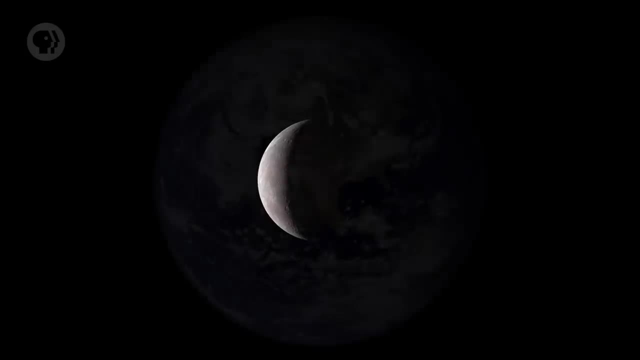 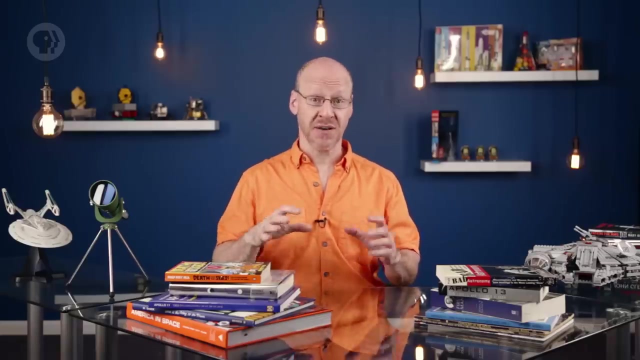 worse, it's a dinky planet, only about 4,900 kilometers in diameter, about a third the Earth's width. One upside to all this is that because it's close to the Sun, its illuminated fiercely and can be pretty bright, even near the horizon, If you ever get a chance to see. it. you really should. It's pretty cool. Mercury's orbit is weird. It has the most elliptical orbit of any planet, ranging from 46 to nearly 70 million kilometers from the Sun. When it's closest to the Sun, it receives. more than twice as much light and heat as when it's furthest. Mercury's too small and difficult to observe to see surface features on it which for a long time made it impossible to figure out how long its day is. Astronomers assumed that the tides from the Sun had locked Mercury's. spin, so that its day was equal to its year, just like our Moon spins once for every time it goes around the Earth. However, in 1965, astronomers used Doppler radar to observe Mercury and directly measure its spin. and they got a surprise: Its day was only 59 Earth. days long, not 88, but that's a significant number as well. To be more exact, the actual length of Mercury's year is 87.97 days, and the actual length of its day is 58.65 Earth days. If you divide those two numbers, you see their ratio is almost exactly two-thirds. 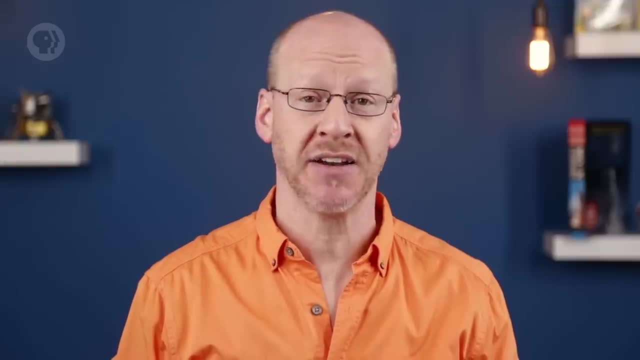 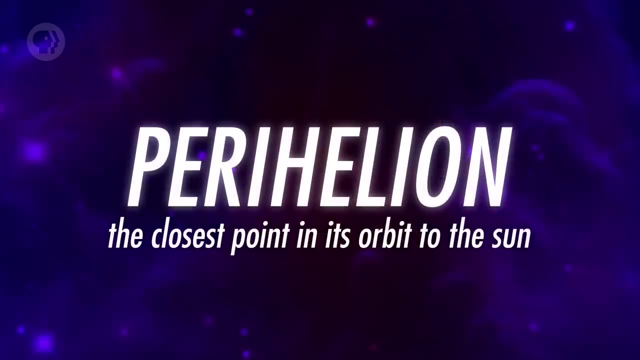 It turns out there's more than one way to tidally lock the rotation of a planet to its orbit. Remember earlier when I said Mercury's orbit is highly elliptical. The tides from the Sun are far stronger on Mercury when it's at perihelion, the closest point in its orbit. 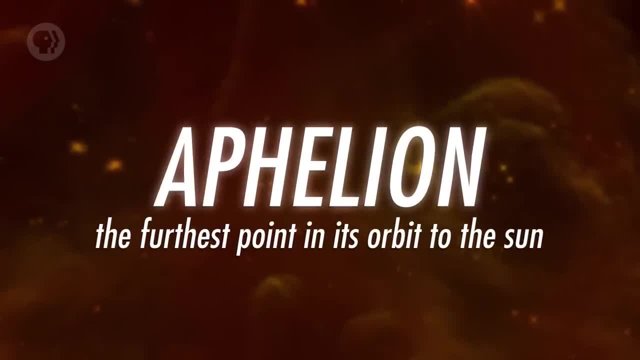 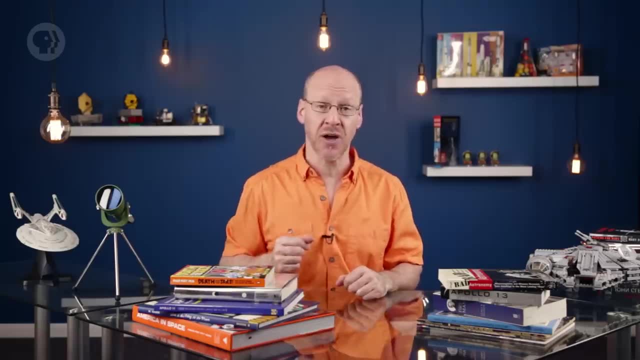 to the Sun than when it's at aphelion, the farthest point in its orbit. After Mercury first formed, tides from the Sun slowed its rotation, just like the Earth's tides on the Moon slowed the Moon down as well. But at some point Mercury's orbit was more 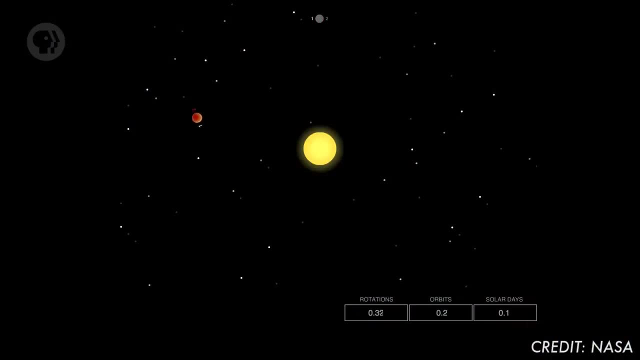 elliptical, Mercury's spin slowed to where it was two-thirds of its orbital period. So at one perihelion pass one side of Mercury faces the Sun. Then 88 or so days later it approaches perihelion again, But it's spun one and a half times and this means 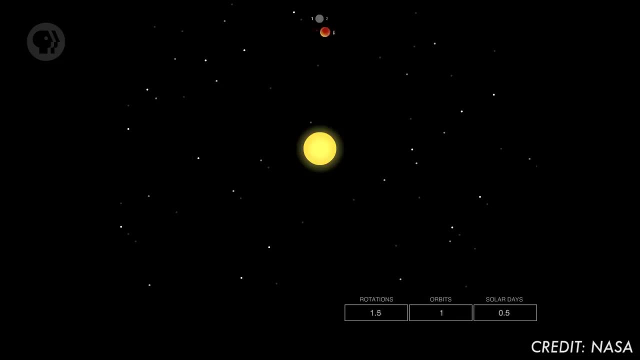 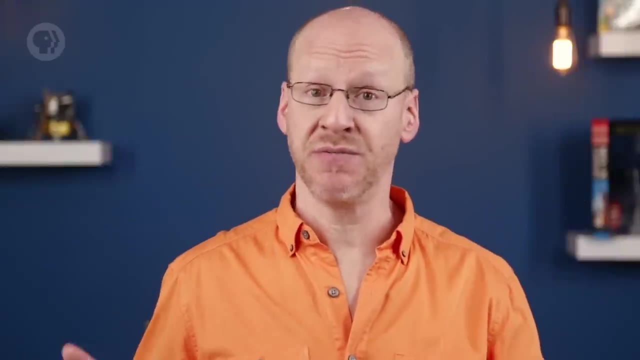 the exact opposite side of Mercury faces the Sun at this closest approach. 88 days later, Mercury is spun one and a half times again and the whole thing repeats. It turns out that's a perfectly legitimate, stable configuration, just like the one-to-one. spin-orbit setup. The way the physics works out tides like simple multiples. They're not always the same. Once the day became two-thirds the period of the year, forced by Mercury's elliptical orbit, the tides stopped slowing it. And things have been that way. 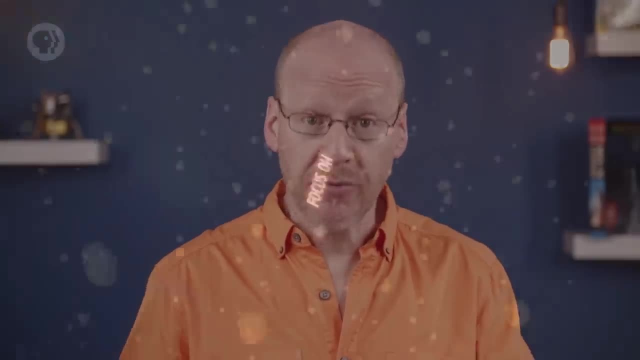 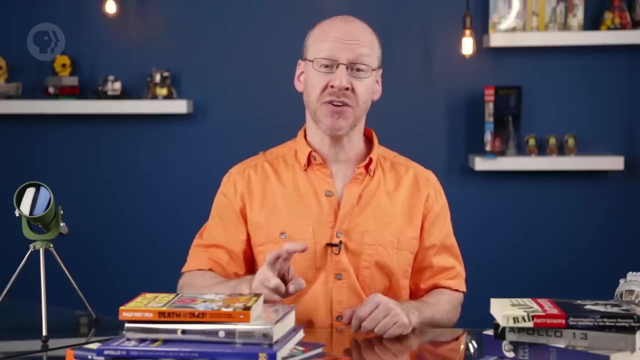 ever since. Mercury's elliptical orbit, together with the two-to-three spin-to-orbit ratio, make for a very, very weird day on Mercury. If you stay in one spot, it takes the Sun two Mercury years, 176 days- for the Sun to go around the sky once. That's because if you're on the side of Mercury facing the Sun at one perihelion, the other side will face it one year later. It'll only be after the second year ends that you're facing the Sun again. 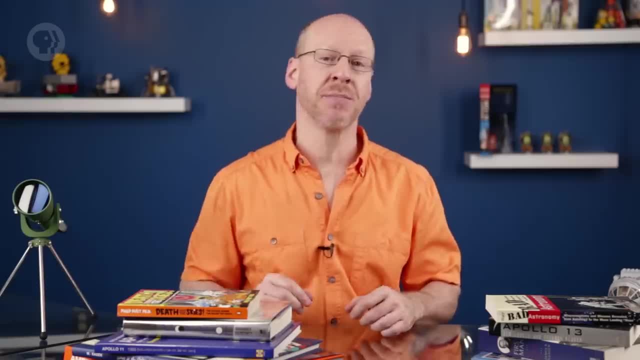 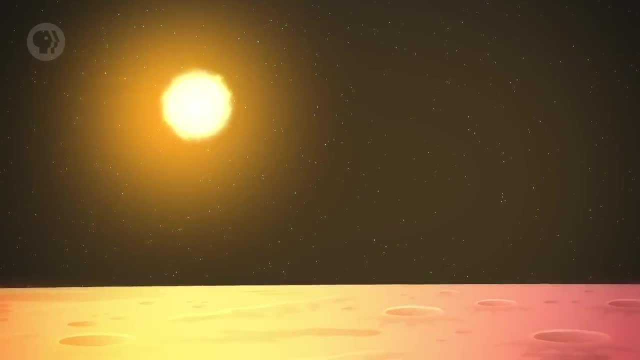 But it gets weirder. Mercury's spin is constant. It doesn't speed up or slow down. However, its motion around the Sun is faster at perihelion than aphelion. At aphelion, Mercury's spin is a bit faster than its orbital speed, so the Sun moves rapidly westward across the 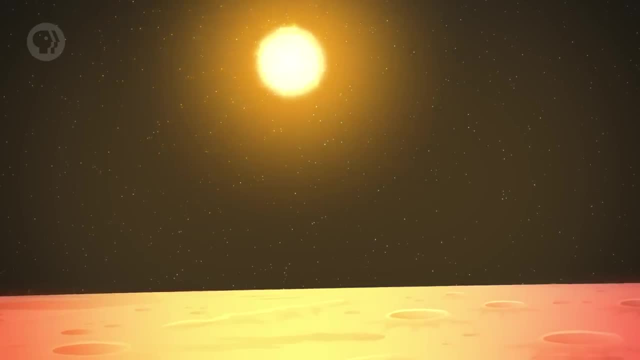 sky, But at perihelion. Mercury's motion around the Sun actually more than compensates for its spin. So the Sun appears to stop in the sky and actually move backwards for a few days. Then, as Mercury pulls away from the Sun, its 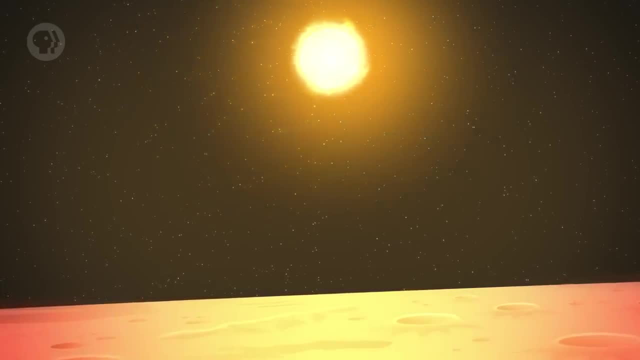 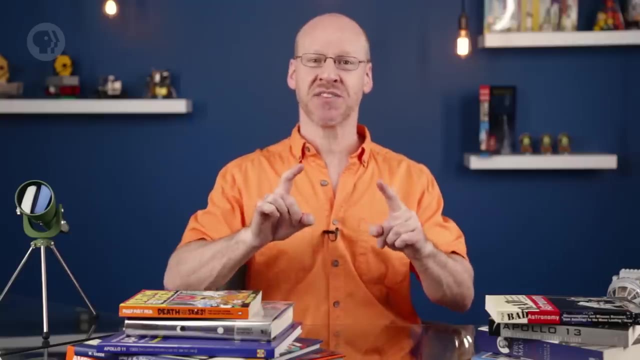 orbital velocity slows down and the Sun starts to move west once again as the planet's rotation dominates. If you're at just the right spot on the planet's surface, this means you could actually watch the Sun rise slow, stop set again, then rise again, And you think time zones on the 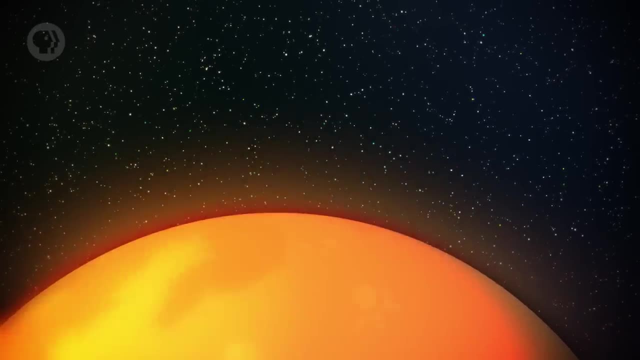 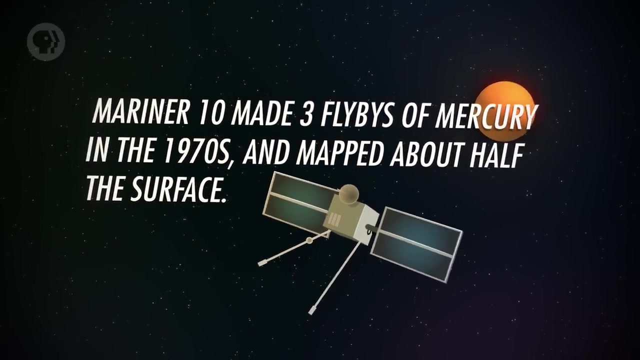 Earth are a pain. Mercury's hard to observe from Earth and much of what we know about it is due to observations from space probes sent there. Mariner 10 made three flybys of Mercury in the 1970s and mapped about half the surface. We learned that it had almost 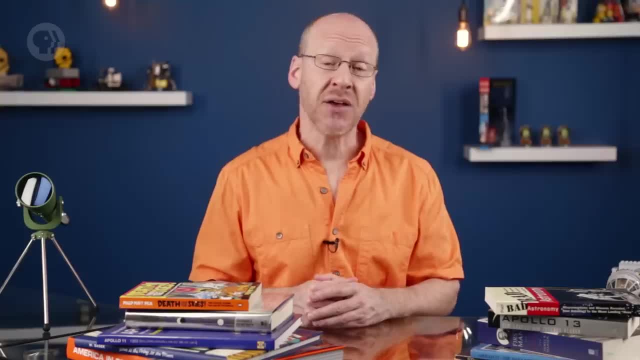 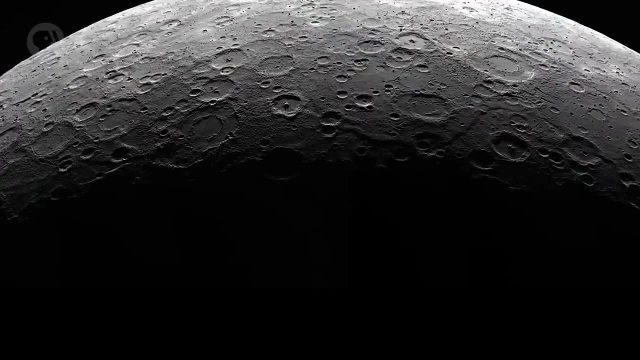 no atmosphere and was therefore unsurprisingly covered in craters. In 2011,, the MESSENGER probe entered orbit around Mercury after making a series of close flybys. The pictures it returned were breathtaking and revealed a world that has seen a lot of. 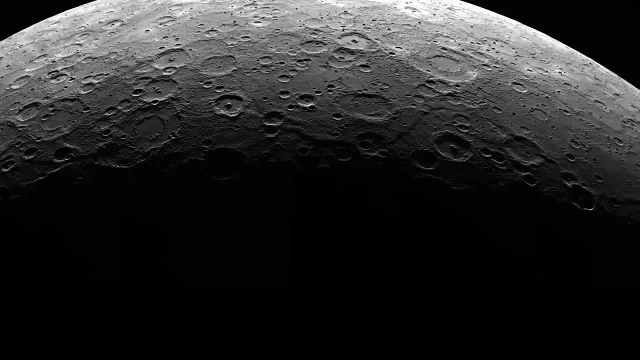 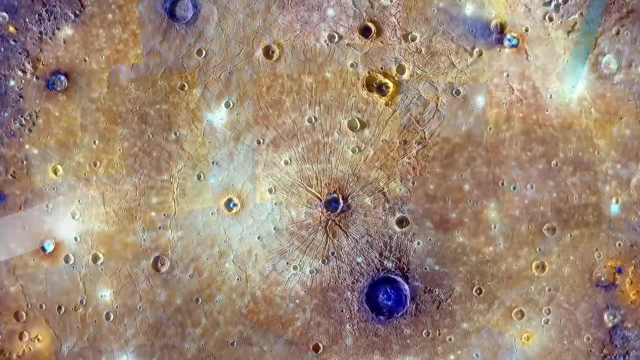 pummeling over the eons. It's covered in craters pole-to-pole, some hundreds of kilometers in diameter. The largest is called Caloris Basin, a whopping huge impact feature 1,600 kilometers across. There are some smoother planes on the planet's surface too, which 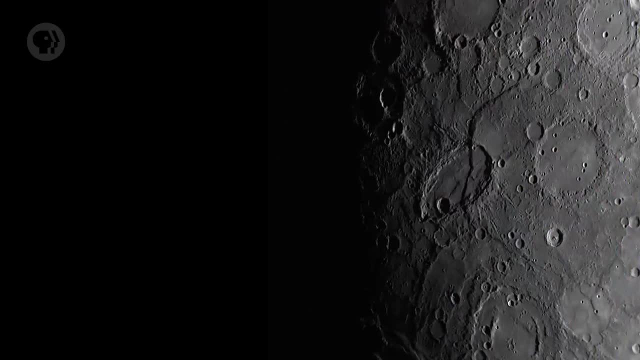 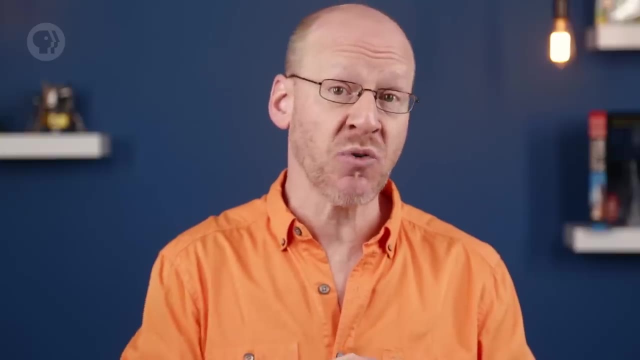 appear to be older than the cratered regions. These planes are covered in cracks, which are called rupes. These are compression folds, like wrinkles on a fruit rind that's dried out. Apparently, as Mercury's interior cooled after it formed, the planet shrank and the 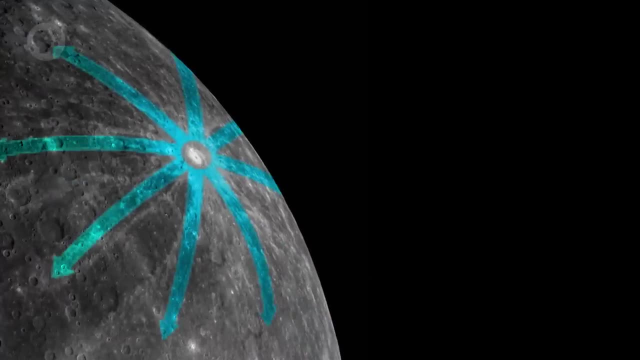 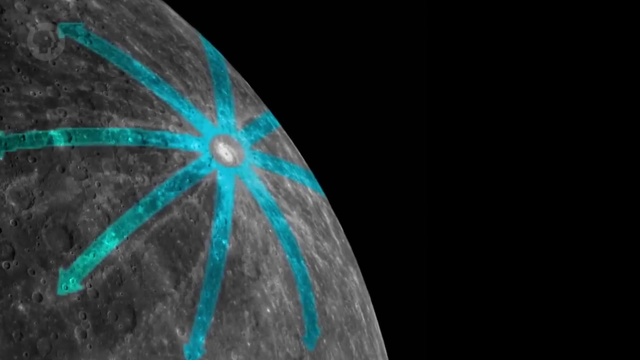 crust cracked as it tried to shrink as well. Several of the craters have extensive ray systems, Like on our Moon. these are formed when impacts fling out long plumes of material that then settle down on the surface. One of my favorite things of all about Mercury — craters are named after artists, Musicians. 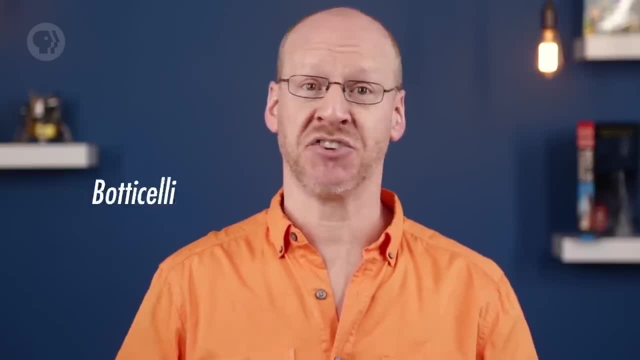 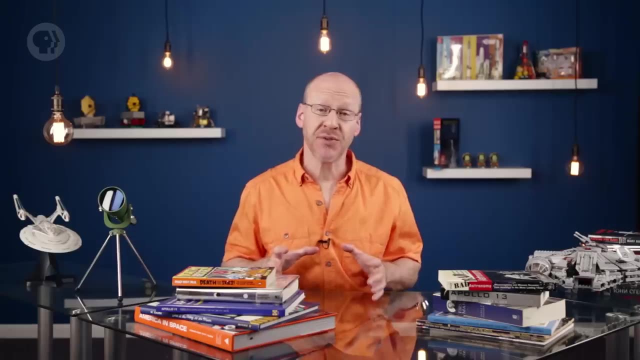 writers, painters and more. So we have craters like Botticelli, Chekhov, Debussy, Degas and Occhio, Sibelius, Vivaldi and Zola. There's even one named Tolkien. Dipping below the surface, we can only infer what Mercury's internal structure is like. 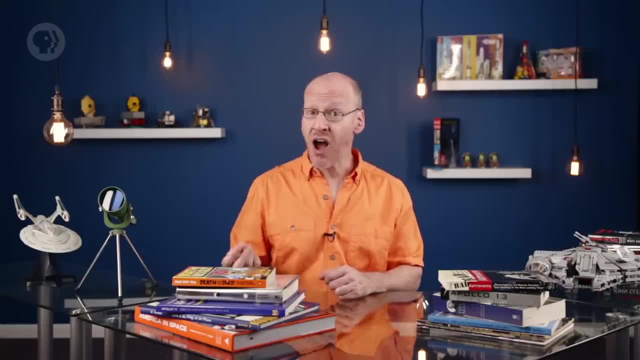 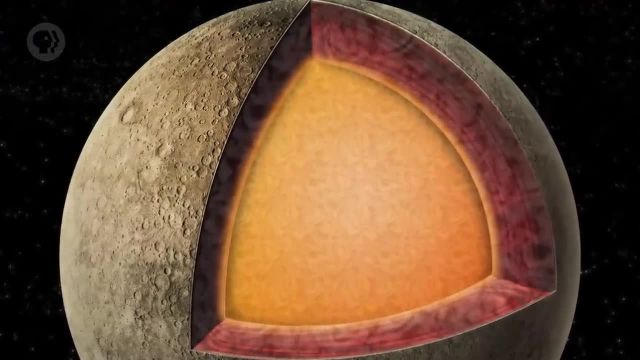 But the planet's dense, nearly as dense as Earth. We know the surface is rocky. so to be as dense as it is, it must have a large iron core, far larger in proportion to the planet than Earth's. Mercury's core may reach three-quarters of the way to the planet's. surface. Why does it have such a high proportion of iron? Mercury may have formed as a larger planet, then got blasted in a huge grazing impact and then became a very, very large impact. It blew away the lighter materials that had risen to the surface, leaving behind 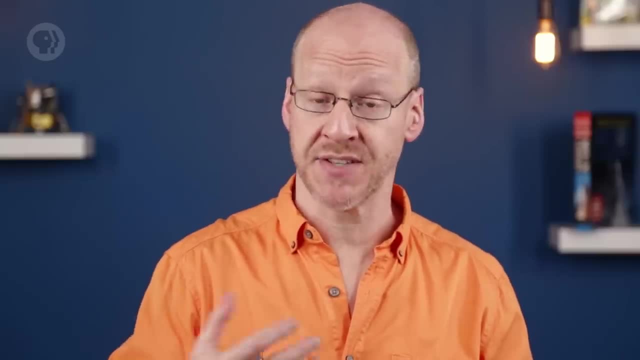 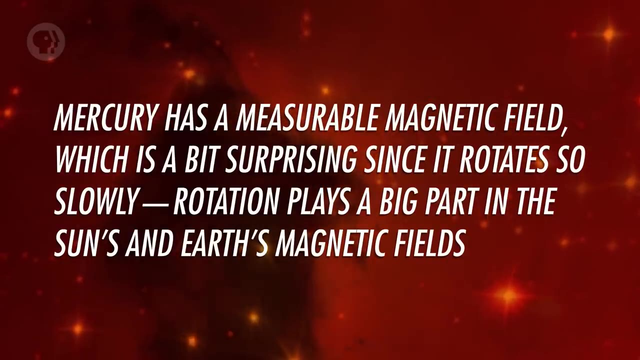 the denser part, Or maybe the heat of the still-forming Sun vaporized the lighter materials off its surface? Mercury has a measurable magnetic field, which is a bit surprising since it rotates so slowly. Rotation plays a big part in the Sun's and Earth's magnetic fields, But that fits with. 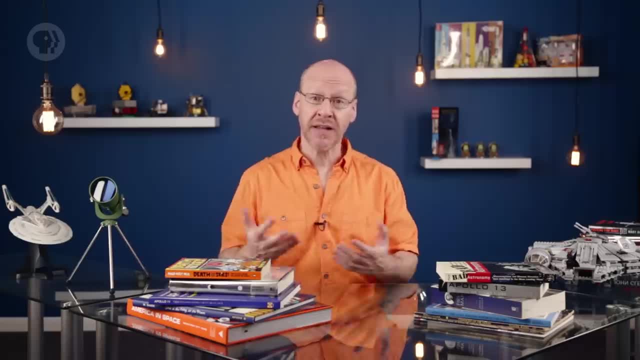 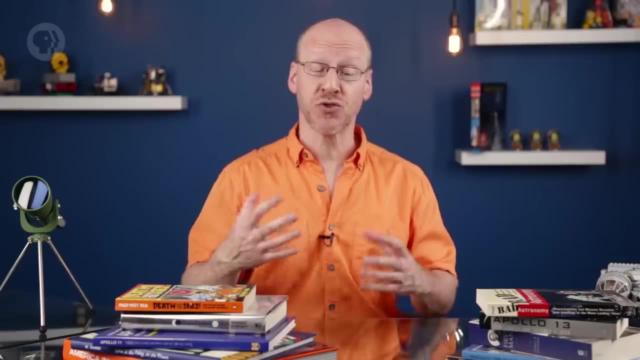 so much of its interior being molten iron. The bigger core may allow for a stronger field. despite its slow spin, It doesn't have much of an atmosphere, but there is a trace of one, mostly due to its magnetic field trapping the solar wind and to material flung up from the surface after. 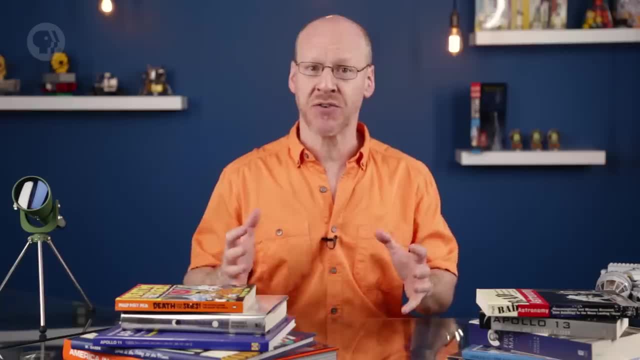 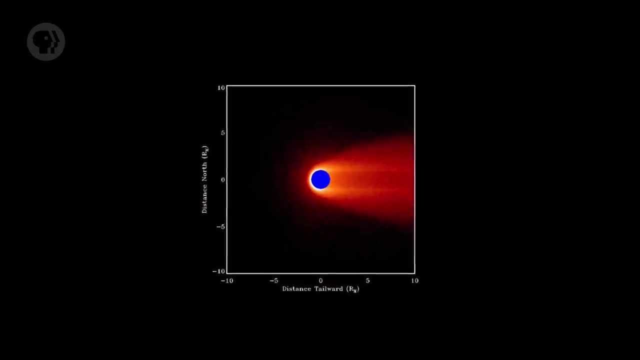 violent impacts from comets and asteroids. A lot of this material blown off the surface escapes the planet and gets blown away by the solar wind and pressure from sunlight. It forms a long comet-like tail that is tens of millions of kilometers long. This tail, 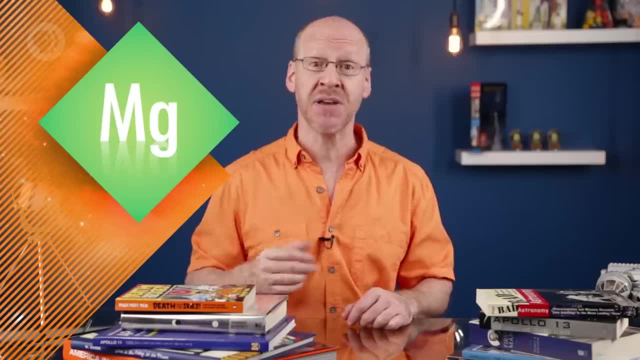 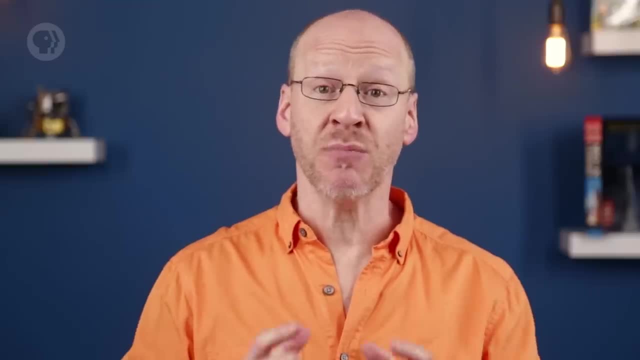 is comprised of elements like sodium, calcium and magnesium, material that's known to be abundant on the surface. Speaking of which, here's a fun fact: Pound for pound, impacts on Mercury are more violent than they are on Earth. Mercury has weaker gravity, so it doesn't pull in impactors as hard as the Earth does.